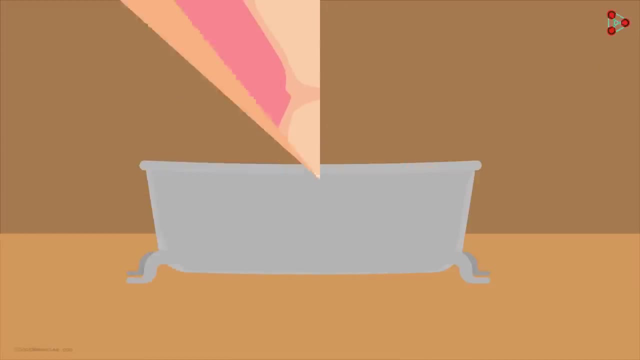 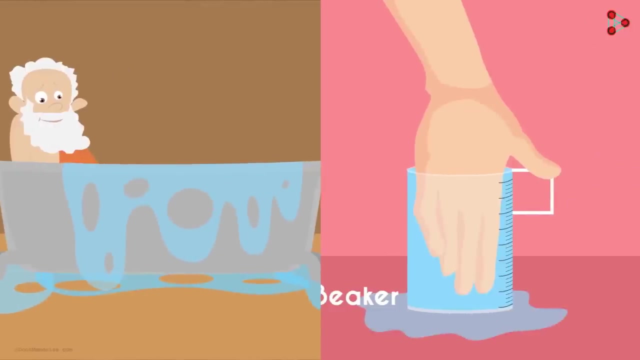 increases significantly. The ancient Greek mathematician Archimedes observed something similar when he got into a bathtub. When he got in, he realised that the level of water went up. In both the cases, you notice that the water is displaced by the object that goes in. 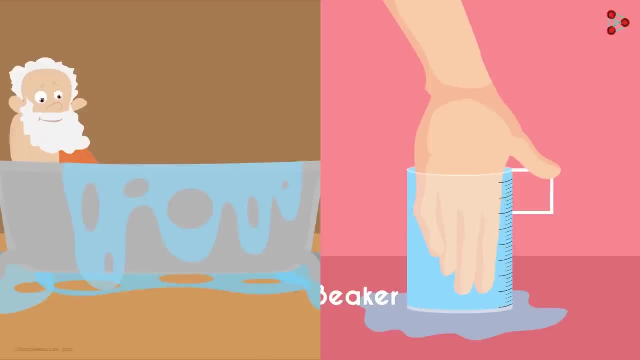 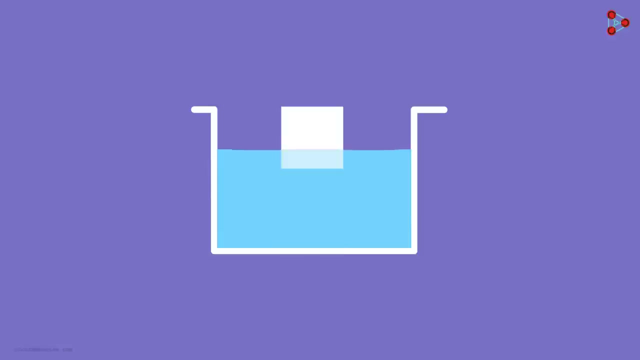 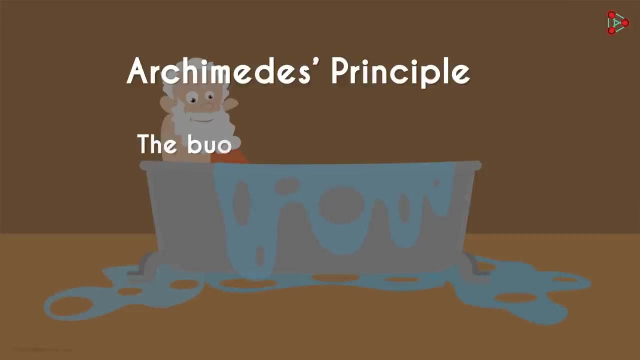 Keep this thought in mind. we will come back to it soon. In our previous videos we have seen that when an object is placed in or on the fluid, the fluid exerts a buoyant force on it which acts upwards. The Archimedes principle goes just one step further in saying that the buoyant force 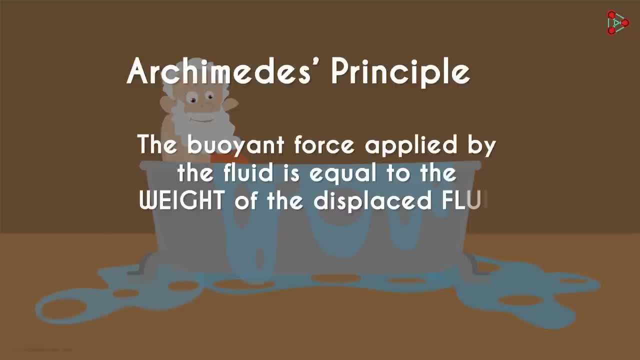 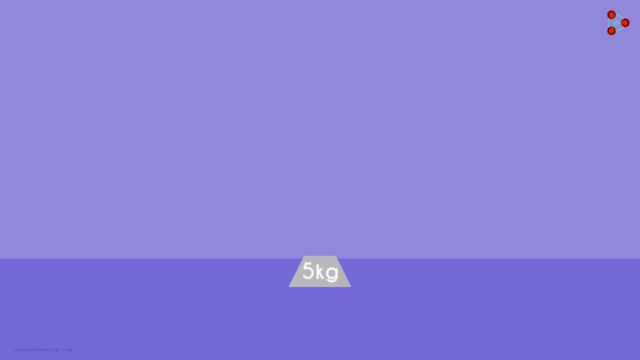 applied by the fluid is equal to the weight of the displaced fluid. We can take a simple example to understand this. Take a 5 kg solid object and suspend it by a spring balance. The balance will read 5 kg. Let this be the first case. 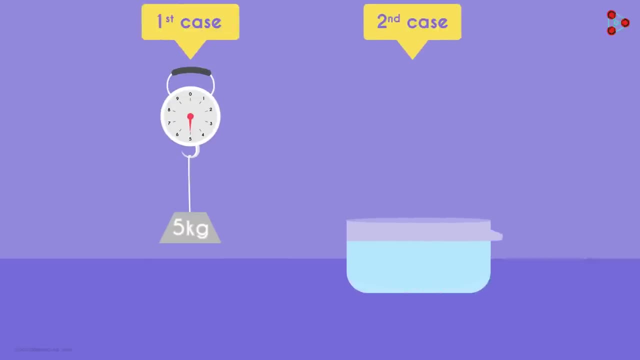 For the second case, take a beaker of water which has a small opening at the top. The water in the beaker is filled right up to this point where the opening is And we keep a small container under the opening. Now slowly lower the solid object into the water and you'll see that the reading will. 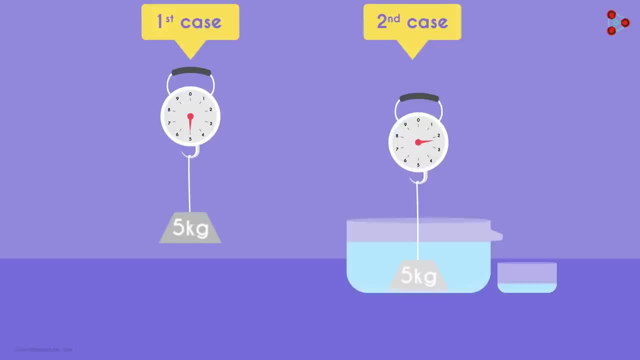 be lower number as compared to the previous case. Why is that? It's because of the buoyant force acting on the object. You'd have also noticed that some water was displaced. Now, in this context, we can say that the weight of this displaced water is equal to the mass. 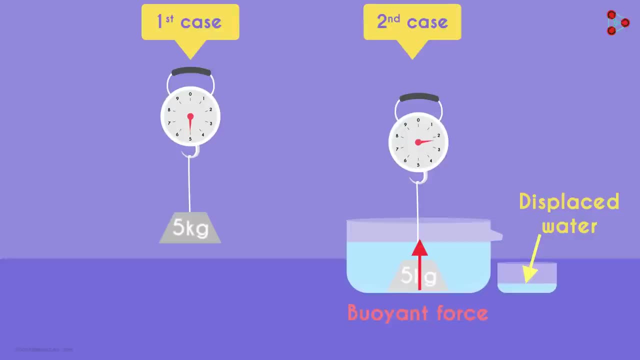 The weight of this displaced water is equal to the mass. The weight of this displaced water is equal to the mass. The weight of this displaced water is equal to the magnitude of the buoyant force acting on the object. That's the Archimedes Principle. 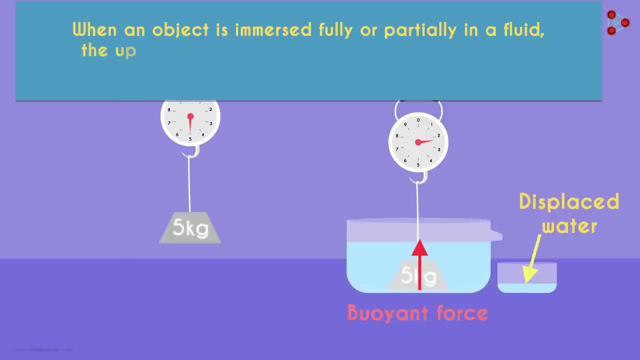 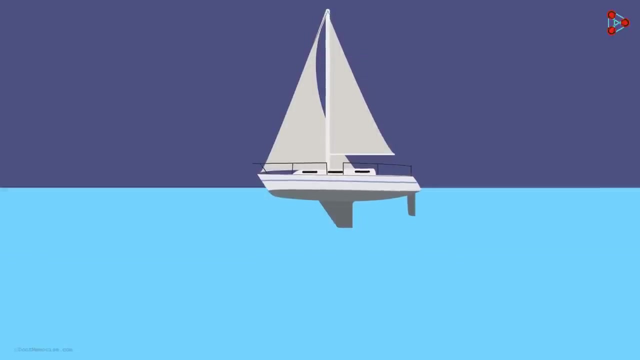 When an object is immersed fully or partially in a fluid, the upward force applied by the fluid on the object is the same as the weight of the fluid displaced by the object. Where is this principle applied? Can you think of examples? How do you think large steel ships float? 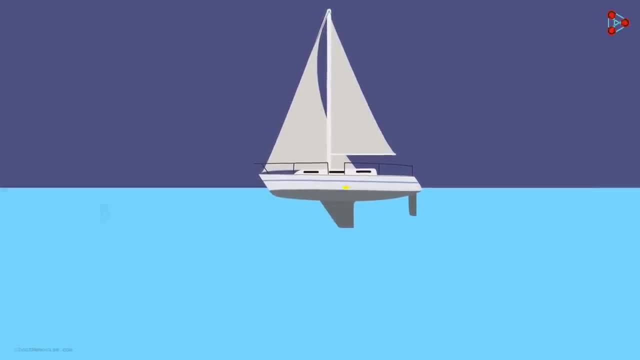 It's simple: If the weight of water displaced by the vessel below the keel is equal to the weight of the vessel below the keel, then everything above the keel will remain afloat. That's because the water too applies an upward buoyant force on the ship which is same as 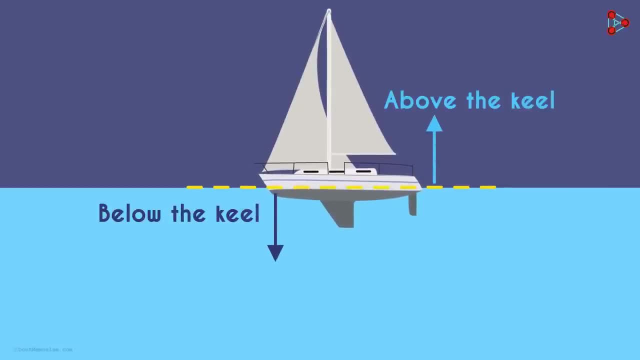 the weight of the water displaced by it. That's because the water too applies an upward buoyant force on the ship which is same as the weight of the water displaced by it. There's just one important concept left in this section, and that's relative density. which we will cover in the next lesson.